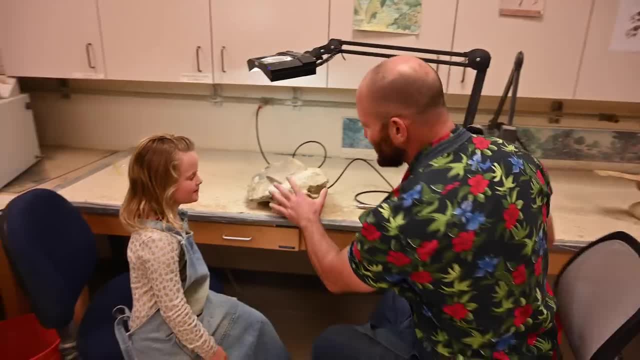 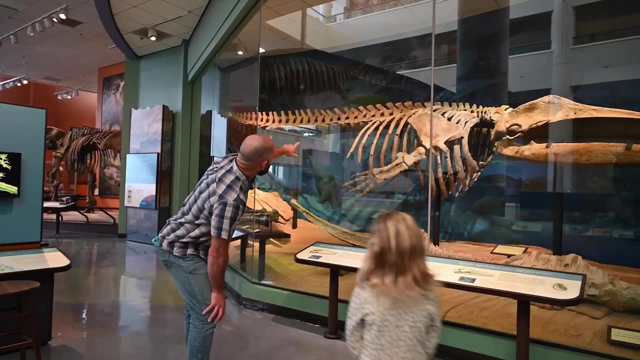 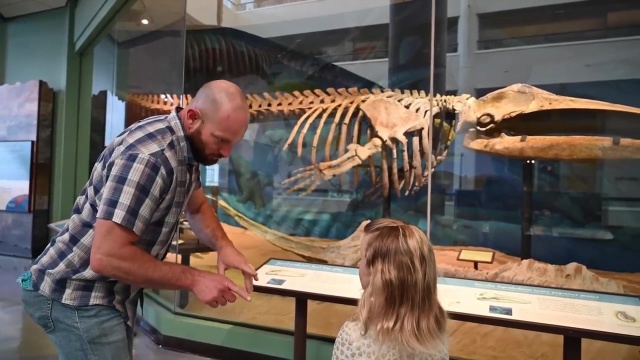 the base of the skull to the bottom of your back, and this right here is a vertebrae from a whale. If we were to remove all the sediment from the fossil the, the whale vertebrae would look something like this: So it has the body vert. 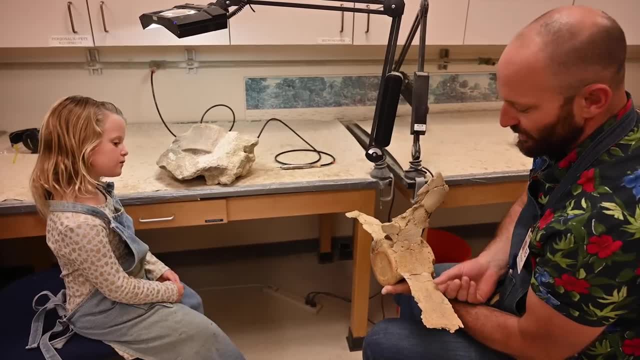 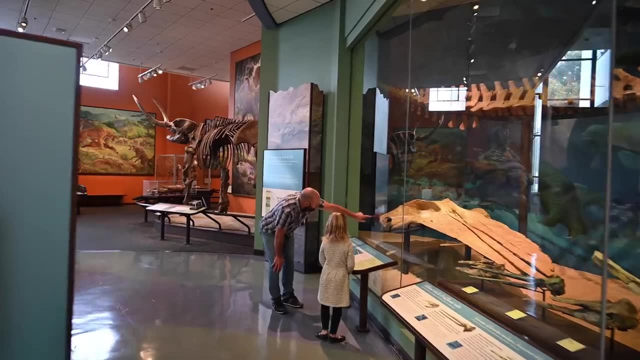 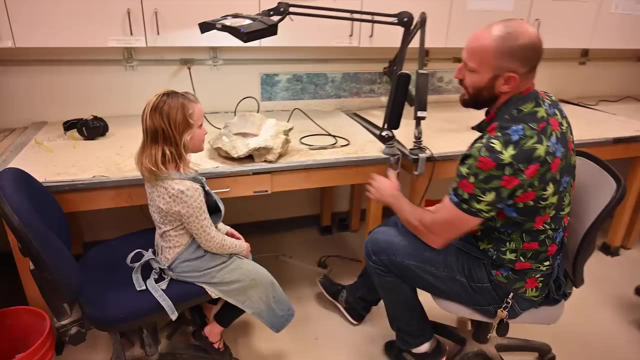 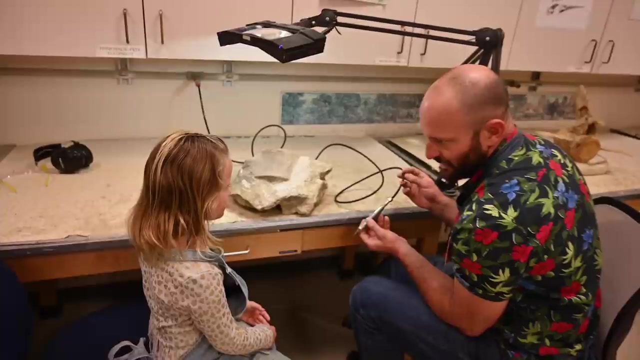 and then these are some transverse processes, and then this is where the spinal cord runs through the back of the whale. So what we're going to do today is we are going to remove the sediment from this whale vertebrae with a tool called a scribe. Now, this is a compressed air. 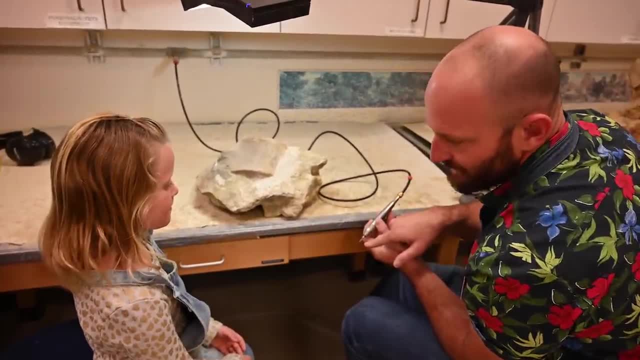 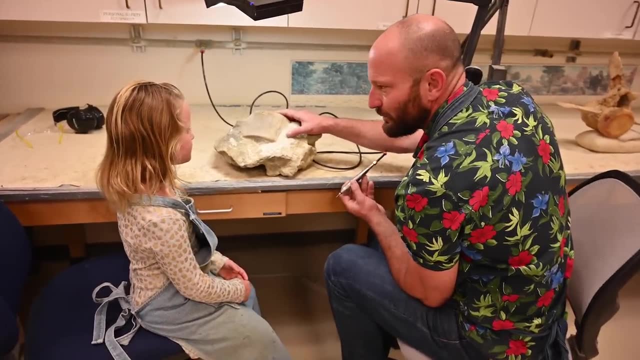 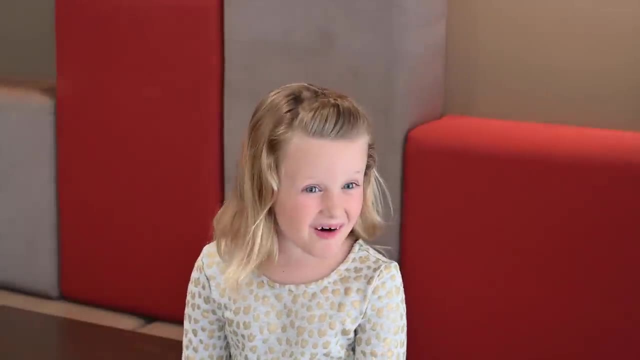 tool. so this little needle right here will vibrate up and down like a little jackhammer and it will remove the sediment from the fossil and we will free the fossil from its encasement inside all this dirt. You ready? I got to clean a whale fossil. 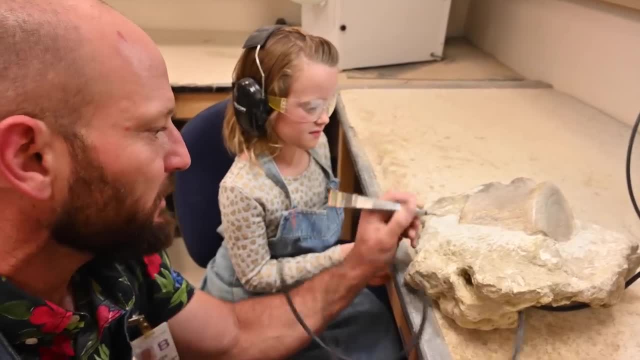 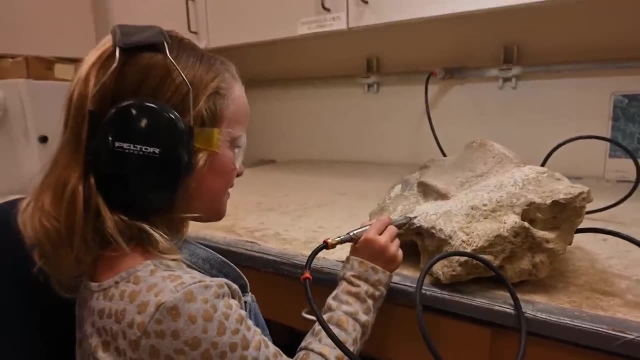 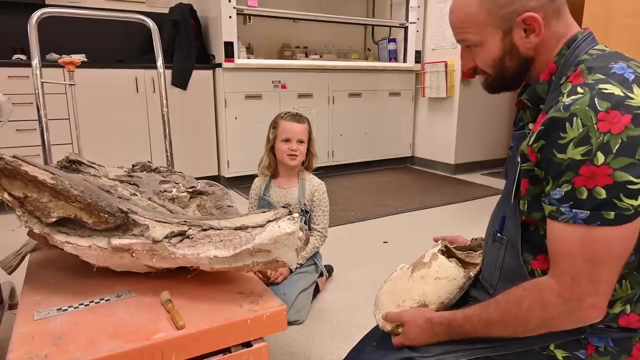 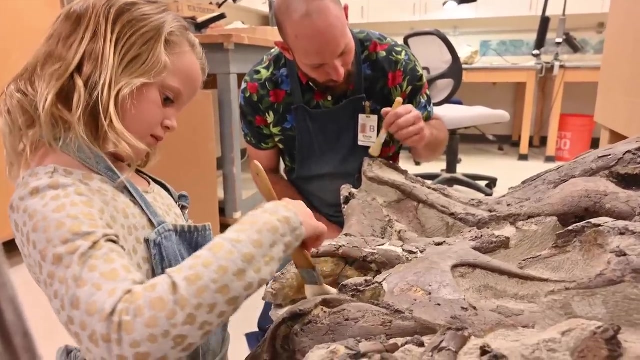 The paleontologist even showed me a real dinosaur bone. Do you like finding them? I do. It's like finding a present that's been waiting for you for millions of years, and I get to sit here and prepare the fossils. I get to clean them up. 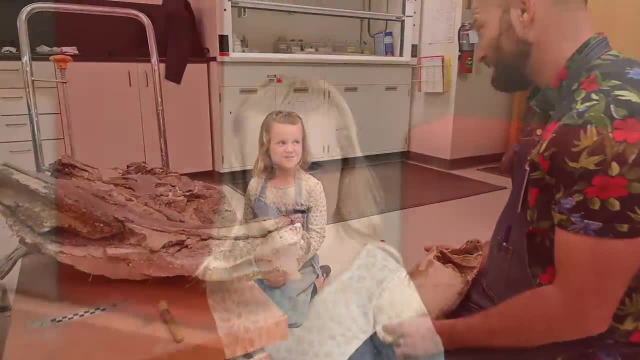 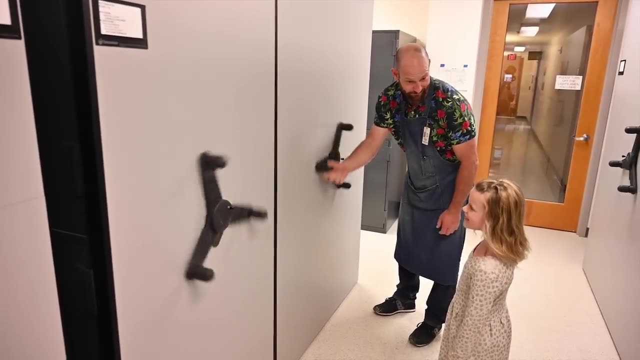 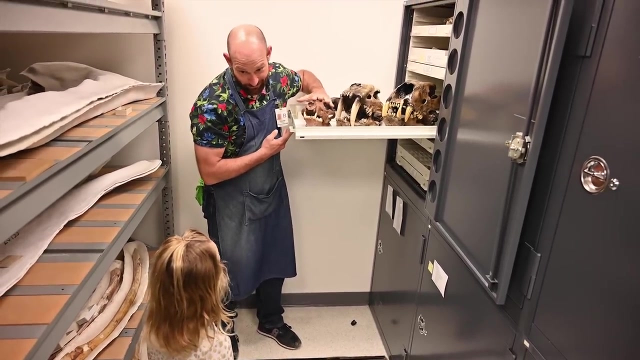 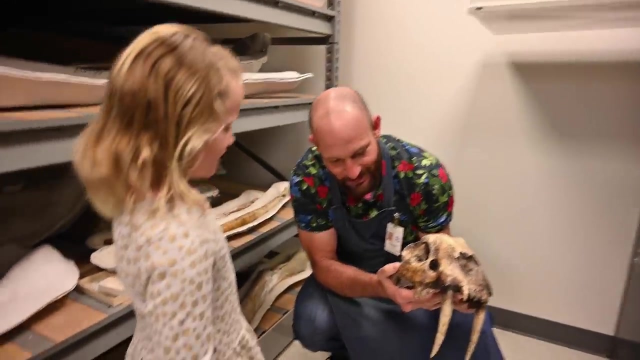 So it's like opening a present. every day, I learned about fossils that lived a long, long time ago. This is where we keep all our fossils: It's the American lion, the saber-toothed cat and the dire wolf. This is the saber-toothed cat. Isn't that cool? Look at those teeth. 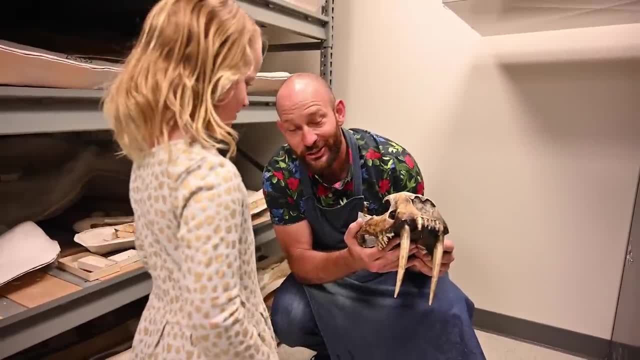 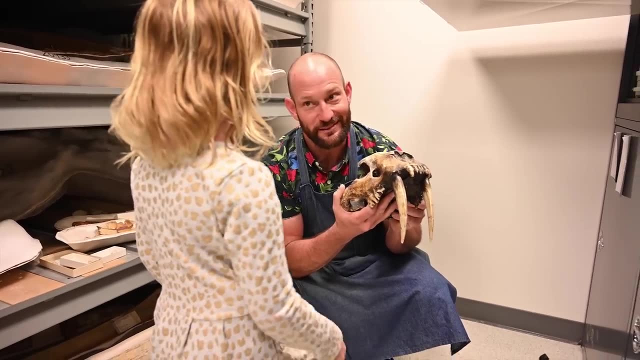 His teeth are like, They're huge. So what do you think this guy looks like? What does this guy like to eat? Plants, Animals, Animals. you're right, Yeah, he likes to eat animals, Like seabirds, Exactly. yeah, So these used to live here in Southern California.